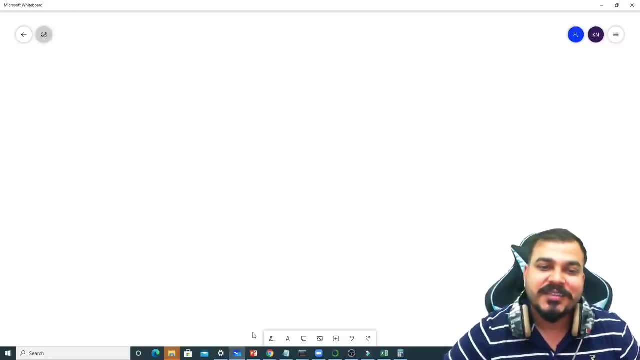 Hello, all my name is Krishnak and welcome to my YouTube channel. So, guys, today, in this particular video, we are going to discuss about application programming interface. Application programming interface, We basically call this as APIs. Okay, this is a very, very important thing, guys, which is called as APIs. Okay, and in this video, I'm just going to discuss with respect to data science. It is very, very handy, You. 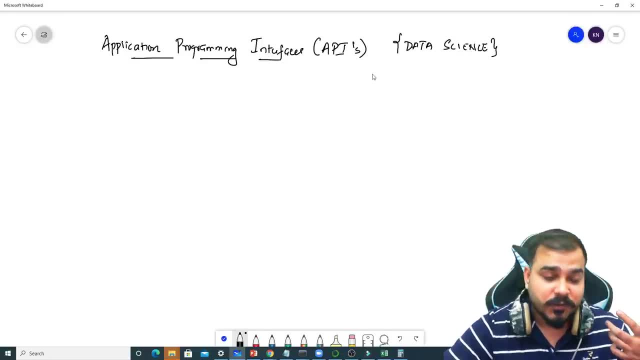 everybody needs to know about APIs. This will be specifically helpful when you're deploying your models into the cloud. Now let's take an application example like Netflix. Okay, Now in Netflix, if I consider some recommendation system, some of the operations like recommendation systems right, Recommendation systems Right. And you have also seen that whenever you open Netflix, every time you know the thumbnail. 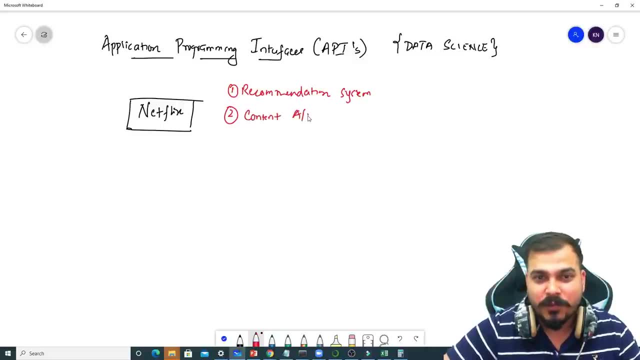 changes. I'd like to say this as content A to B. Content A to B, That basically means every time or after some amount of time, you know, you'll be able to see that images of the movies gets changes and people if they like that specific image and they may probably click that particular movie and get it. Now let's first of all discover about recommendation system. How probably can recommendation work? Now a user who is actually using Netflix, right? Who is actually using Netflix right? 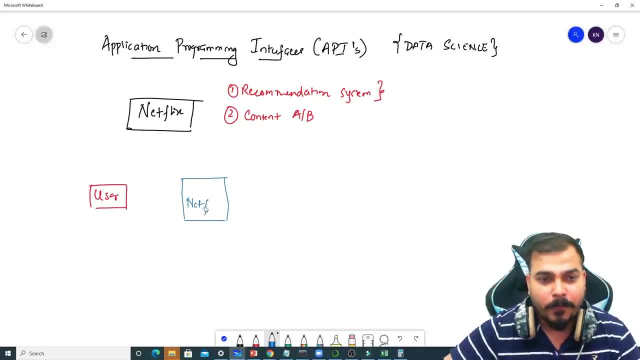 So this is his Netflix app application. Okay, Now, in this particular Netflix application, what does the user do? This application probably may have some of the information stored in this. It can be his user history, It can be his personal information, like a name, age, all those things, right, It can be different kinds of informations And, based on this, probably there may be a model which takes this information like the user. 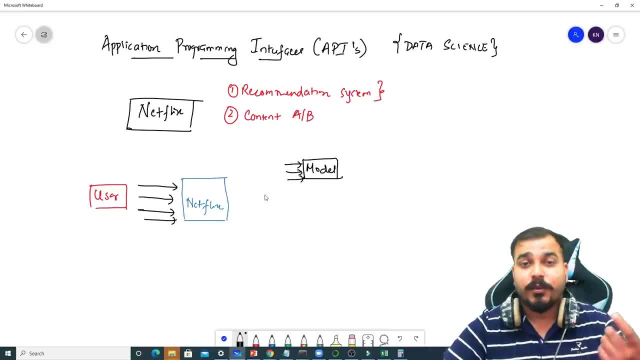 history. what kind of genre is basically, what kind of movies that person like, whether it is an action movie, whether it is a different kind of movie, whether it is a comedy movie, and apart from that, he may also have some of the features like age, and all based on this, this move, this model will. 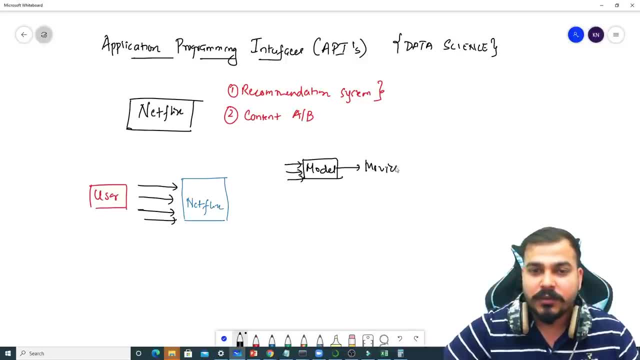 be recommending what kind of movies needs to be recommended to the, to the user, right? so this is the model. this is the model. this model is usually hosted in cloud, so suppose i have a cloud. just see guys, different types of cloud, probably netflix, i. i don't know which cloud they use, but i think 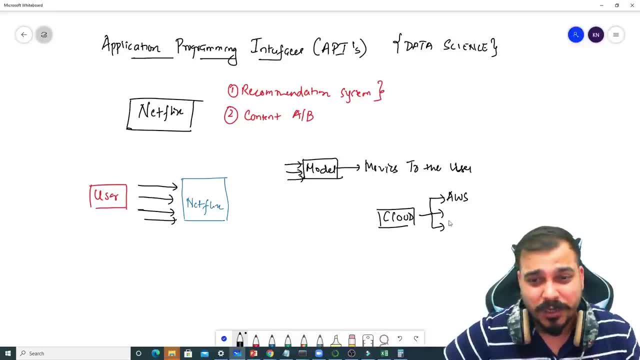 they may be using aws. i'm not sure about it. you can again verify it, google it. there are different clouds, like azure aws, but most of the companies uses this two amazing cloud because there are a lot of functionalities as such. now, when this model is hosted in this particular cloud, it is exposed. 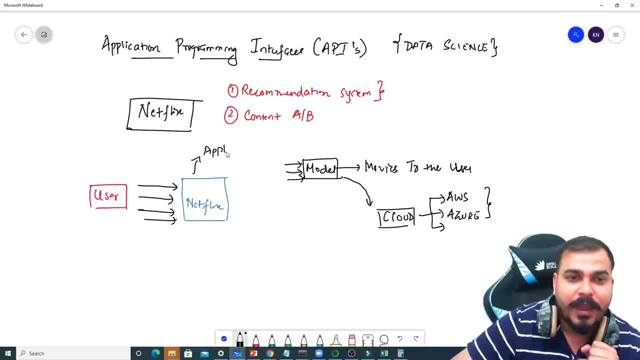 probably. this is my netflix application. right, this is my application mobile application. it is exposed to this, this netflix application, in the form of apis. now, what is this apis? this apis is nothing but application programming interface, so what it does is that, whenever the user is basically 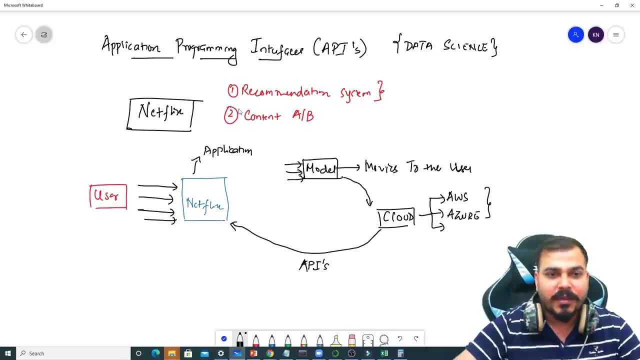 uh, refreshing netflix or his opening after some time. it may happen in such a way that all this information of the user may be taken by this application and then, at the first instance, this information is sent to the cloud where the model is basically hosted, this model, 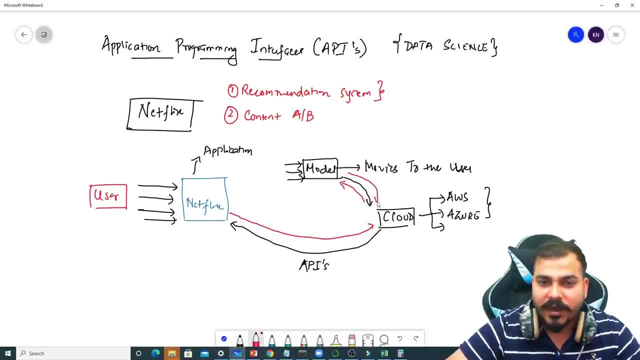 will get the input and, after this, this model will provide a response and this response will, in turn, be provided to the netflix application. then this the front-end developer. with respect to the request that they are getting: they may display that specific movies in front of the specific movies. 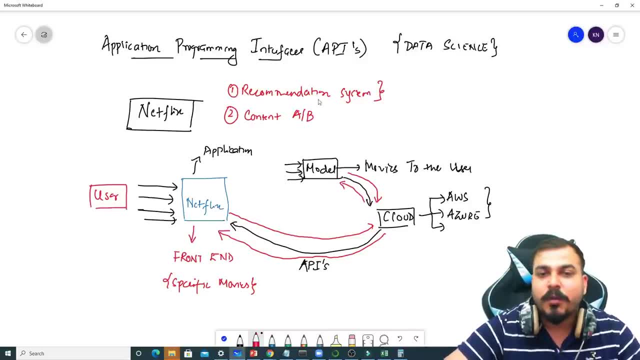 in front of the user right now. how did this model do the production? this model may be have trained in machine learning algorithms. it may be trained in, uh, deep learning algorithms, right. it may be trained in different types of algorithms, right, by using some different techniques. it may be, uh. i've also created a playlist on 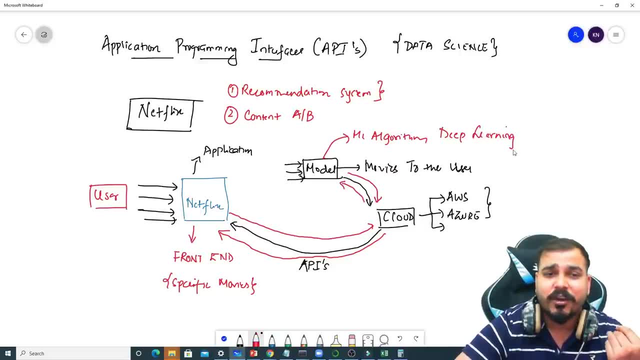 recommendation systems like what are the different kind of machine learning or deep learning algorithms that is basically used now. this api is what it does see whenever we are passing this information. this information will be passed as a post request. right, it may pass as a post request. a post request may be. i may create a json file. 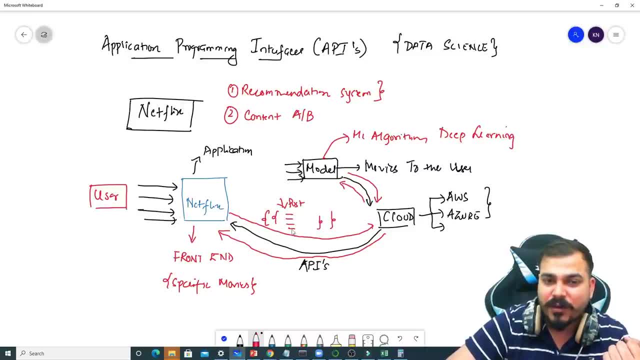 create a json request. in this, all the user information will be there in the form of key value pairs. once this is passed to the model, the model based on this particular input will provide some kind of response right, and this response in turn is parts to the front-end application. this. 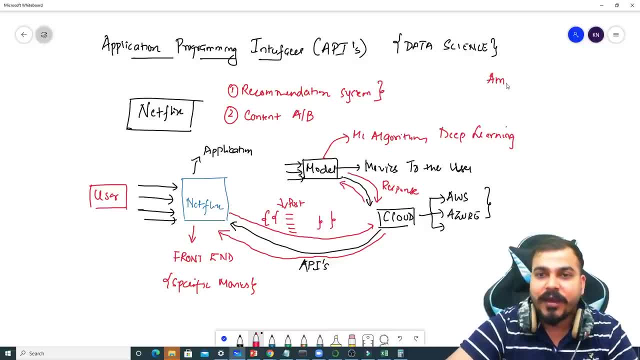 here i've taken an example of netflix. probably i may also have an amazon- amazon in website or web application, right? i think you have seen that mobile app of amazonin. that also may be a front-end application. anything can be a front-end application. right, and remember: in cloud, in cloud. 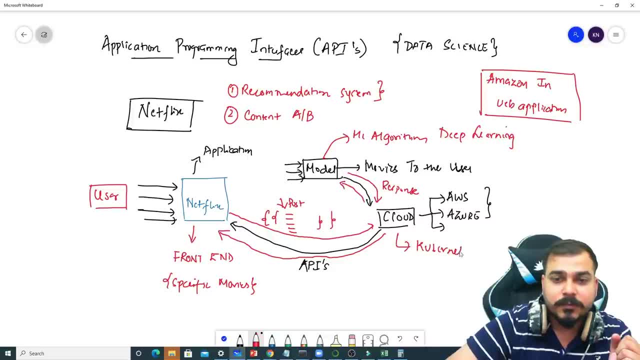 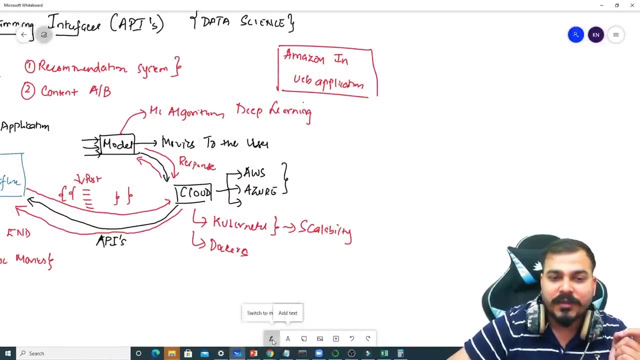 there are the users of kubernetes and docker's for containerizing it. for containerizing it, this is basically used for scalability. that basically means in the cloud. in the cloud, not only one model is basically hosted. there may be- specifically, if i take an example of netflix right, there may be. 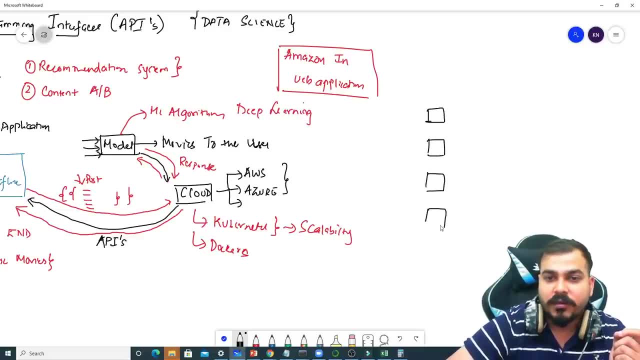 thousand models like this which is basically hosted. this model may be hosted based on regions. it may be hosted based on different different countries. probably a usa country. usa country may have some specific models, some specific thousand models right. india may have, or asian countries may have some specific model right, but india has a huge 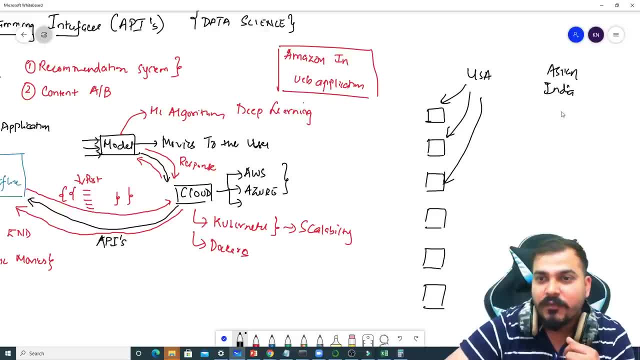 people. i mean india has a huge population who use in netflix for india specifically. they may have a different set of models. you know, based on the user history they will be able to do this recommendation now within this particular model. you know this request will be going to continuously. 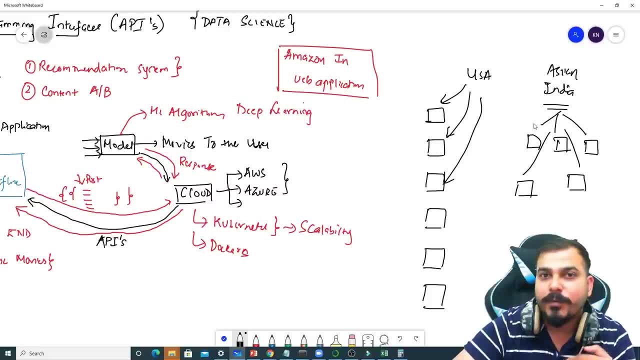 to many models as such, right how which model should be providing it, providing the answer. it depends on the the number of requests that are coming right. it depends on the number of requests that are coming. so that is why the scalability factor can also play a very, very important role. 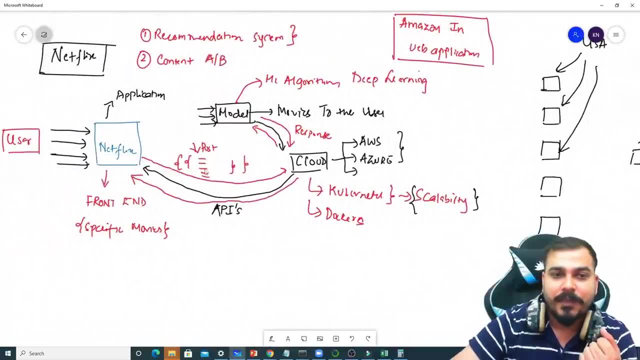 but now, what is the main thing about here is basically about this api, how we are communicating with the model and how the model is basically giving the response right and with respect to this particular model, you may be requiring a lot of information like keys, right, the user names. i i mean some type of password, and keys will be there where, so that they'll be able.